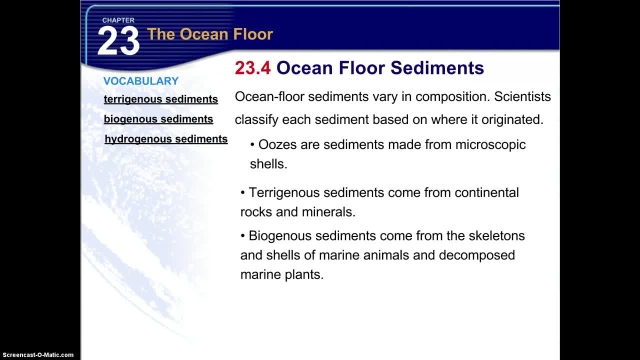 Now, the remains of these abundant marine organisms precipitate into the ocean floor as siliceous ooze, which then forms the sedimentary rock known as chert. Now, this process is similar to the one by which calcareous oozes lithify to form chalk. Now, both chert and chalk are often found with marine limestone deposits. 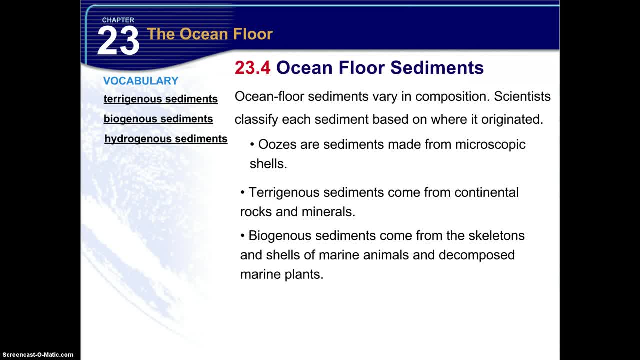 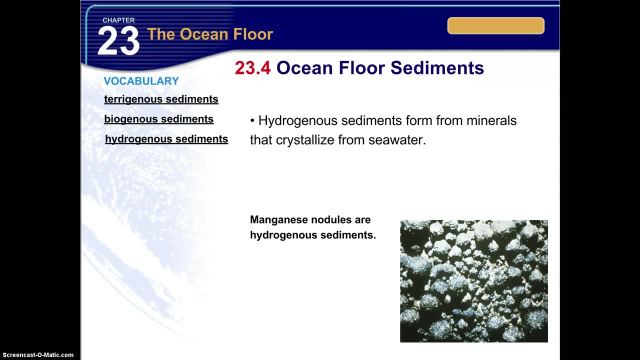 Chert was an important raw material for prehistoric humans. Its fine texture allowed it to be chipped to form sharp edge tools and weapons. Now hydrogenous sediments form from minerals that are crystallized from seawater. Now we have something called a manganese nodule. Now this is a type of hydrogenous sediment that was actually very, very important and still is important. 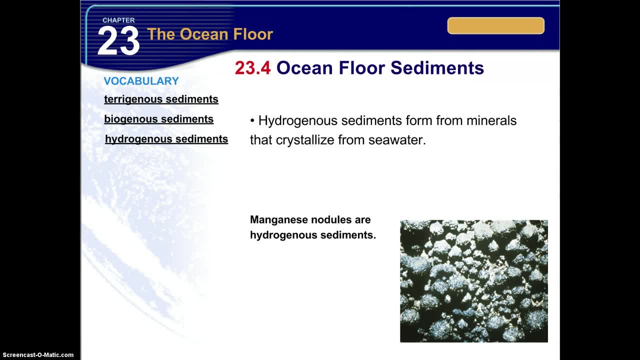 in supporting the idea of there was once a sea, a shallow sea, on the surface of Mars, Because guess what? We found, these manganese nodules on the surface of Mars, And their nickname is blueberries. So if you ever do research, they might be called blueberries as well. 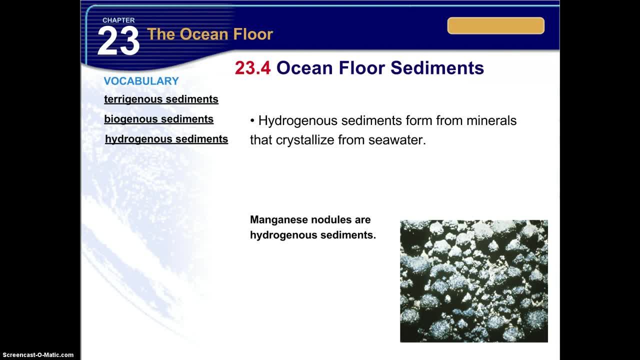 Now exploring the deep sea can be very expensive and dangerous, But the unique organisms, magnetic records and industrial resources available on the ocean floor are very, very significant Now. they often hide a portion of Earth's hydrosphere, biosphere and geosphere. 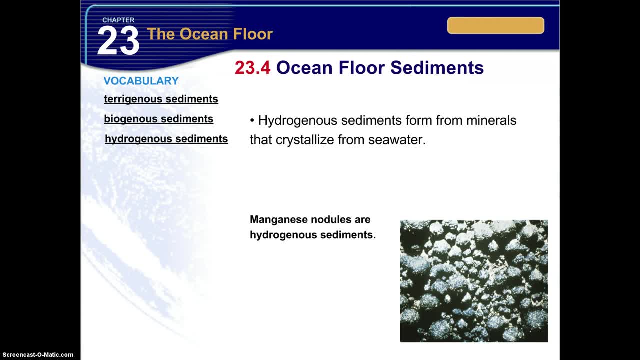 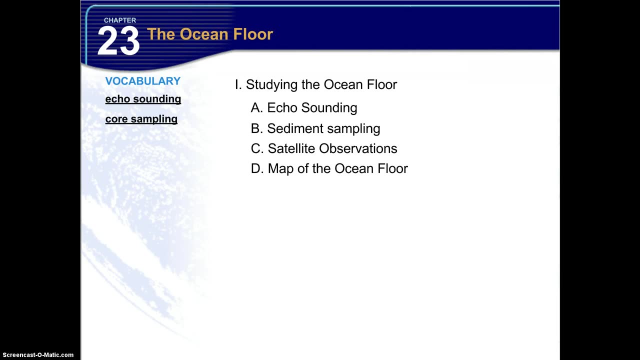 And as one of the least explored domains of our planet, there are many scientific discoveries waiting to be made. still about the deep ocean floor. Overall, in Chapter 23, we started studying the ocean floor: echo-sounding sediments, sampling satellite observations and mapping the floor. 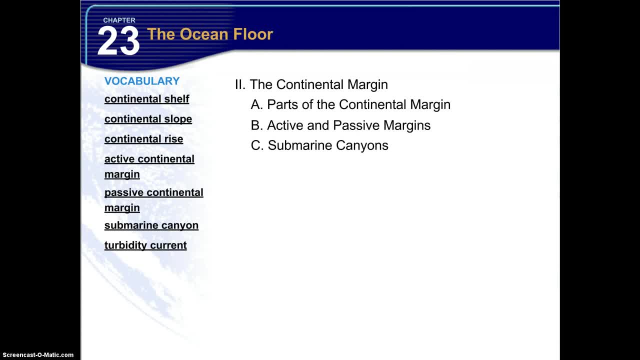 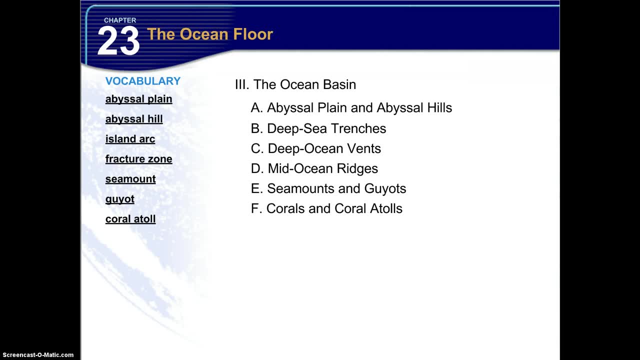 Then we walked through the continental margin, the parts of the continental margin, active versus passive, and talked about submarine canyons and turbidity currents. Now the ocean basin, abyssal plain, abyssal hills, deep sea trench, deep ocean vents, mid-ocean ridges, seamounts and gout corals and coral atolls were in the Section 3.. 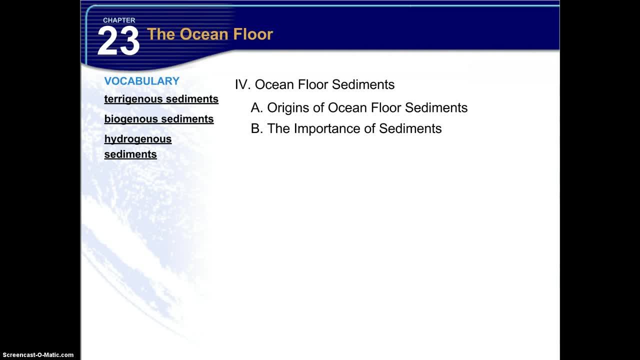 And then, finally, we have origins of ocean floor sediments And the importance of sediments. That's it for Chapter 3.. And